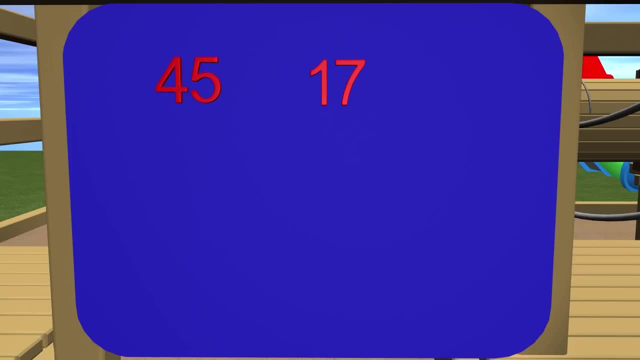 got off the first bus stop. How many students are left on the bus? To get started on this problem, let's first line the numbers up correctly. If we look at the 4 in the tens place, we need to remember that this represents 40, since it is in the tens place. The same goes for: 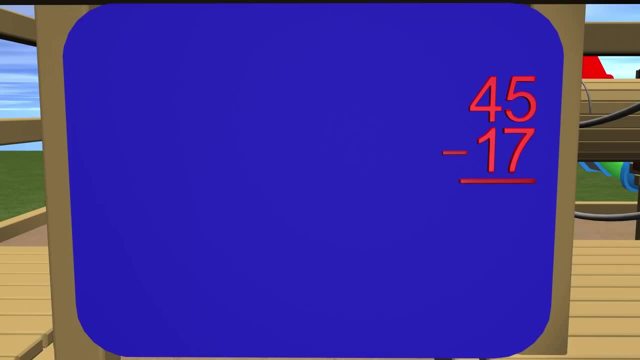 the 1 in 17.. This 1 represents 10 and it is helpful to remember this as we are working the problem. Now that we have the numbers lined up correctly, let's represent these numbers using our place values. To get 45, we need 4 tens blocks- 10, 20,, 30, 40- and 5 ones blocks 1, 2,, 3,, 4, 5.. So 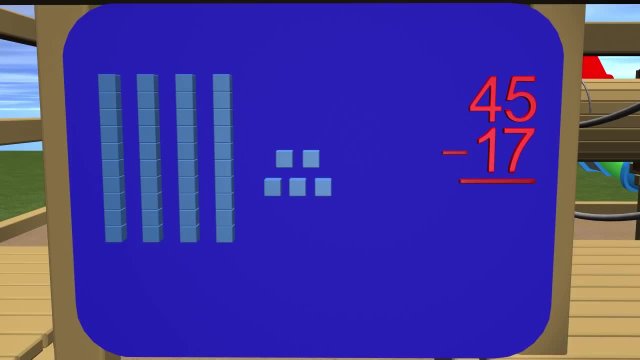 here we have our 45 blocks and we know we need to subtract or take away 17 blocks. So let's start with subtracting the ones. How many ones do we need to subtract? We need to subtract 7, so let's do that. 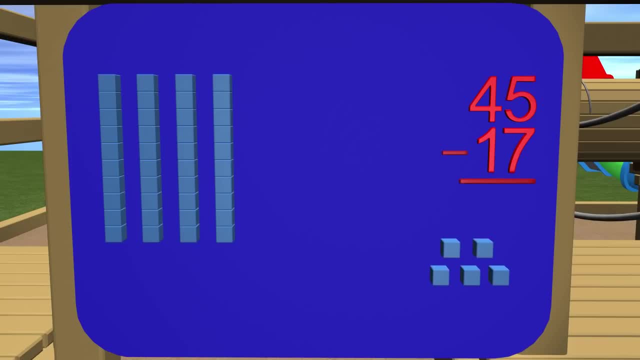 1,, 2,, 3, 4, 5.. Wait a minute. We can't take away 7 ones because we do not have 7 ones to take away. To solve this problem, we need to regroup. To regroup, we need to trade one. 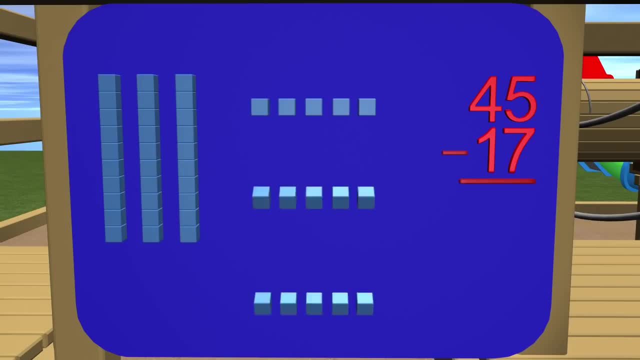 of these tens blocks for 10 ones. Now we no longer have just 5 blocks, We have 15 blocks now. Now we can take away 7.. How many ones does that leave? Let's count and see: We have 3 blocks: 1, 2, 3, 4, 5, 6, 7, 8.. Let's put the 8 under the ones place. Next we need: 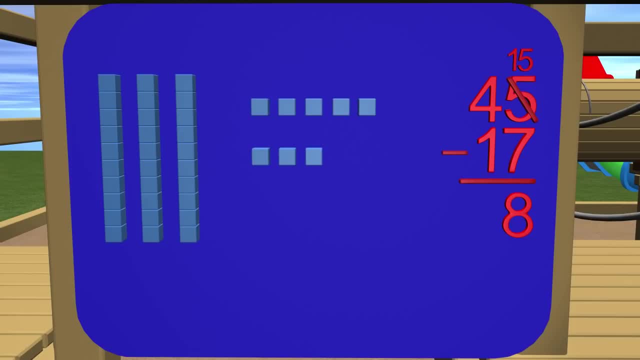 to count the tens place. But wait, We're supposed to have 4 tens blocks, but there are only 3.. Why is that? Oh right, We had to trade a tens block for 10 ones. Let's change this 4 to a 3.. Now how? many do we need to subtract from 3? Right, Let's subtract 2.. How many blocks do we need to subtract from 3? 1, 2, 3, 4, 5,, 6, 7, 8.. Let's put the 8 under the ones place. Next we need to count the tens.